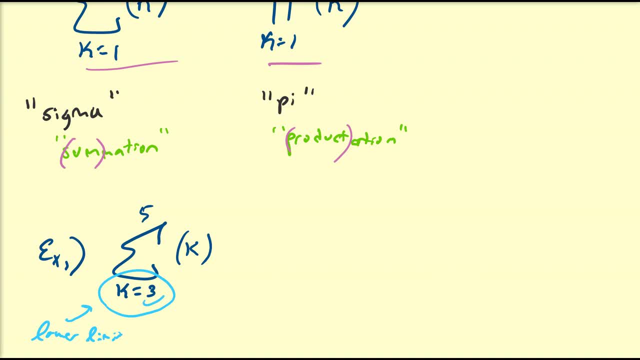 referred to as the lower limit. in particular, three, Five is usually referred to as the upper limit. k is sometimes referred to as the index of the sum, and usually that letter is in the expression to the right hand side. So pretty much what this says is: we're going to replace k with all of the. 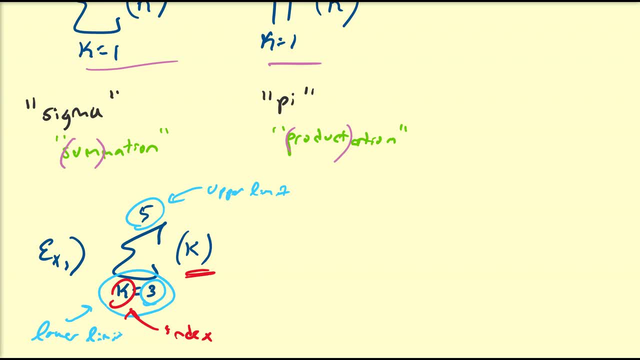 numbers from three to five, and we're talking natural numbers here, and then we're going to add them up, So this is going to be equal to. so replace k with three, that's going to be three plus, and then we're going to increment that by one, so four. then increment that by one to five. 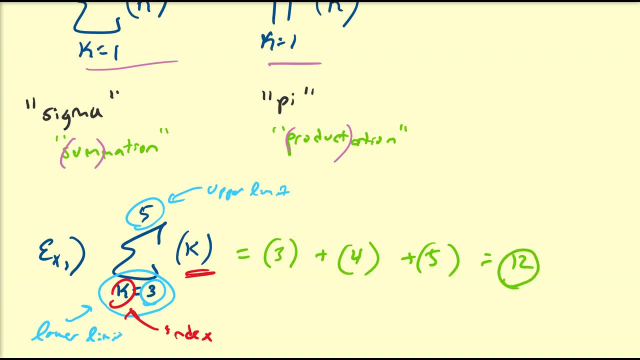 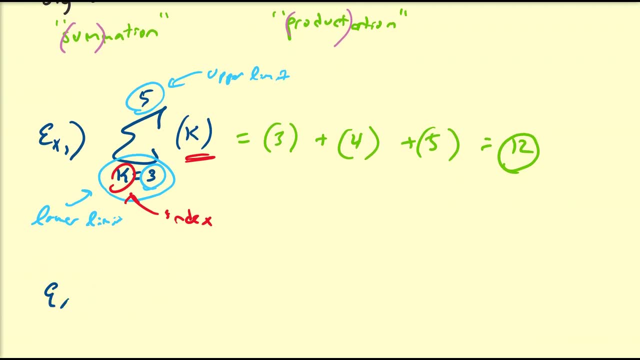 So we have three plus four, which is seven plus five, which is equal to twelve. Therefore the sum from k is equal to three of five, of k is equal to twelve. Let's do another example. Suppose we have the sum from k is equal to zero to two of k squared. So the same thing applies. 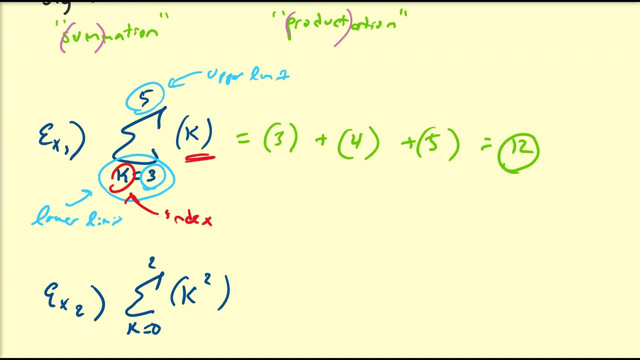 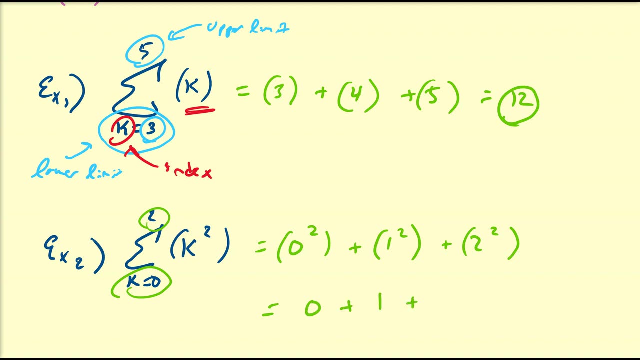 we're going to replace k with all the numbers from zero to two, and then we're going to add up those terms. So this is going to be zero, squared plus one, squared plus two, squared. Notice, we go from zero to two. So this is going to be equal to zero plus one plus four, which is equal to five. 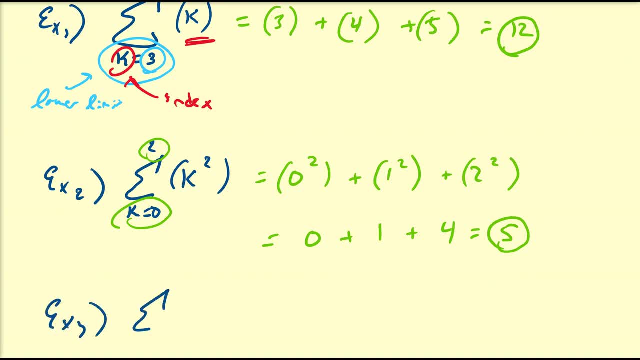 So another example suppose we have: the sum from k is equal to one to two of one divided by k. So same thing applies. we're going to replace k with all the numbers from three to five. so this is going to be one over one plus one over two, which is the same as one plus one half. 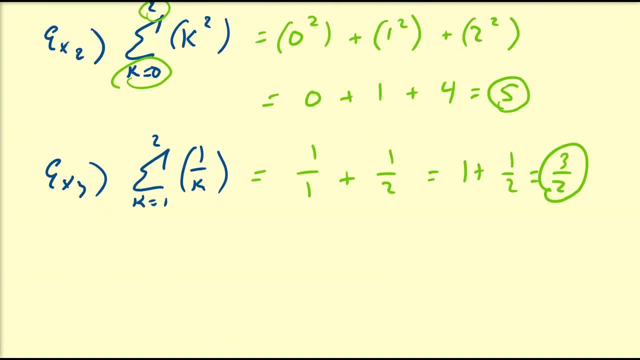 which, as we know, is three halves. So another basic example suppose we have the sum from k is equal to zero to ten, of negative one to the power of k. So we're going to replace k with all the numbers from zero to ten. so this is going. 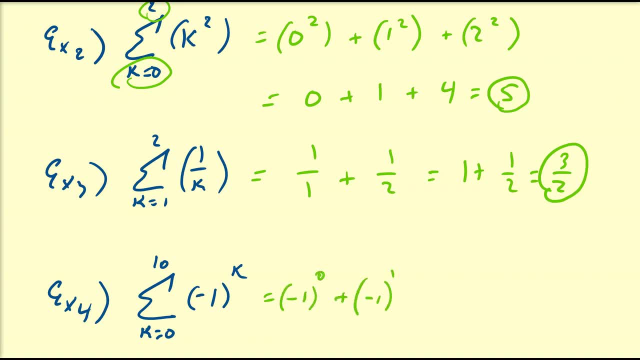 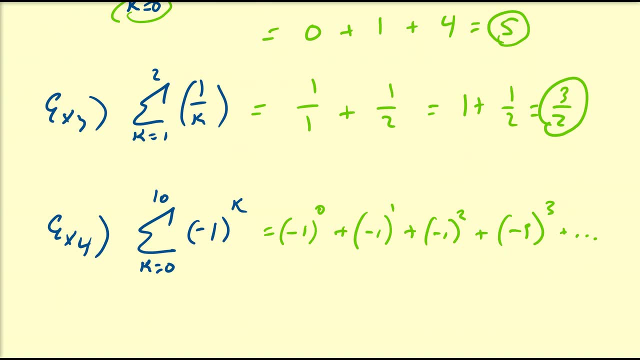 to be negative one to the zero plus negative one to the first plus negative one to the second plus negative one to the third, plus all the way down to- let's go down a few terms- say, negative one to the eighth plus negative one to the ninth plus negative one to the tenth. 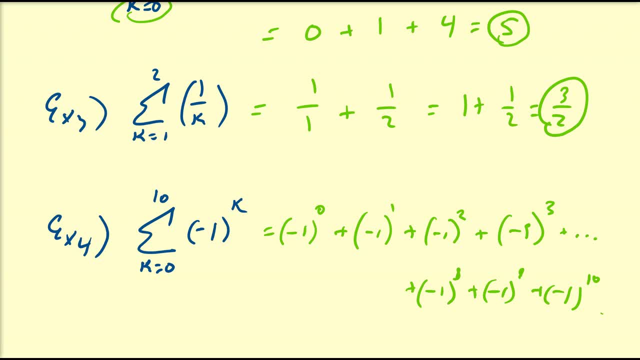 So, as we know, negative one to an even power is going to be one, so this is going to be one, and negative one to an odd power is going to be negative one. So one plus negative one are going to cancel into zero. So the same thing is going to apply here. So two and three. 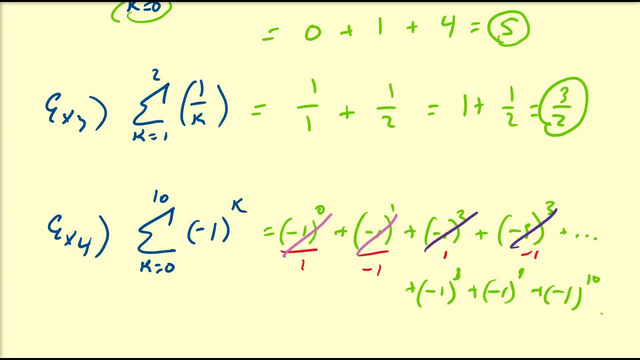 it's going to be one and negative one, so those two terms are going to cancel Notice. we're starting with an even and then an odd, even, then an odd. So eight and nine and all the numbers in between are also going to cancel out with each other, and then we're going to just be left with this. 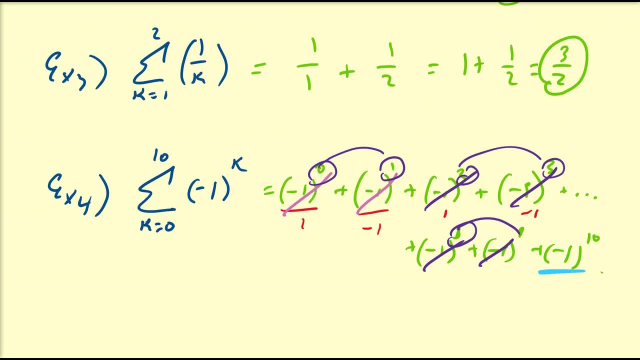 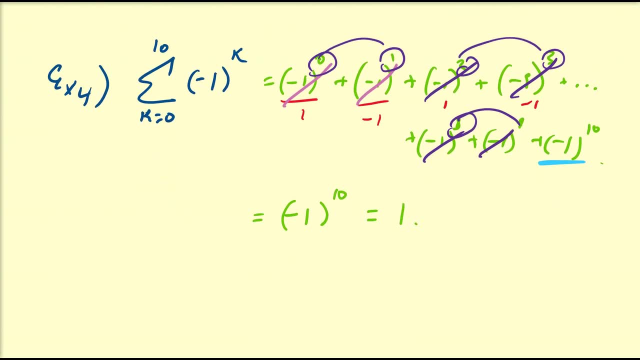 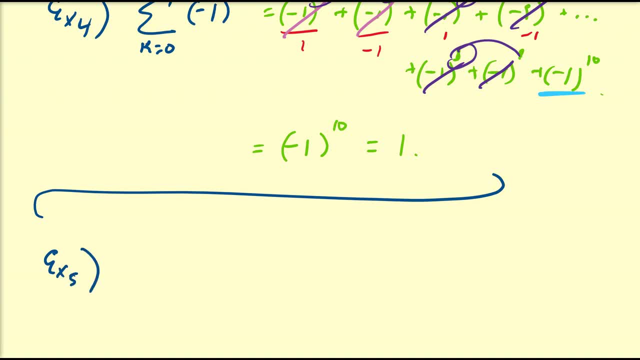 representation. So let's look at a double sum. So the sum from j is equal to zero to three of the sum from k is equal to four, or k is equal to zero to four, And the expression we're going to sum over is j plus k. Some people will not write. 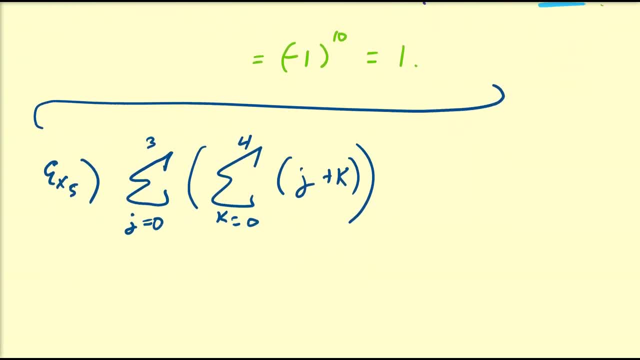 these parentheses, but I'm just writing them here for clarity. So we're going to be focusing on the internal sum here and we're not going to really go into details and properties and tricks and shortcuts. We're just going to go about it in a very intuitive way. So we're going. 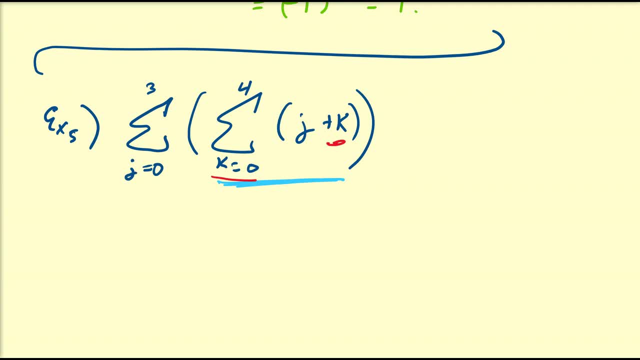 to replace k with all the numbers from zero to four, and then we're going to add up those expressions. So this is going to be equal to the sum from. j is equal to zero to three of. so we're going to have j plus zero plus j plus one plus. 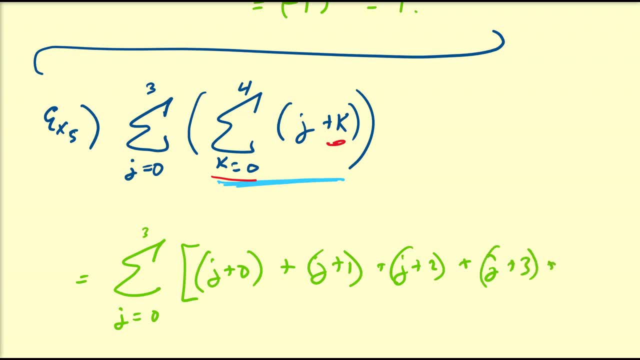 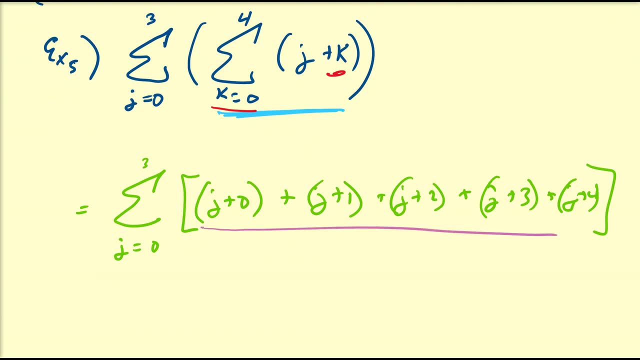 j plus two plus j plus three, plus j plus four. Let's simplify the sum in the middle just to make things a little bit clean. So the sum from j is equal to zero to four. So we have one, two, three, four. five different j's here. So we have five j plus zero plus one is one plus two is three. 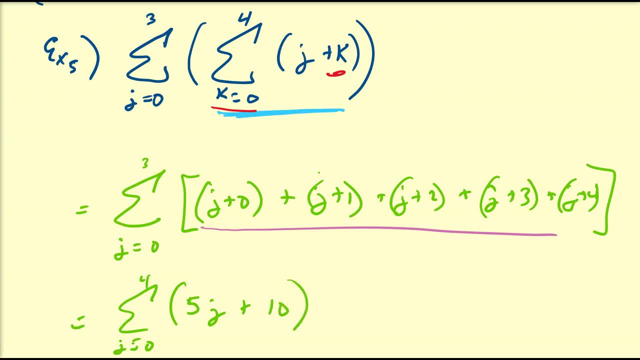 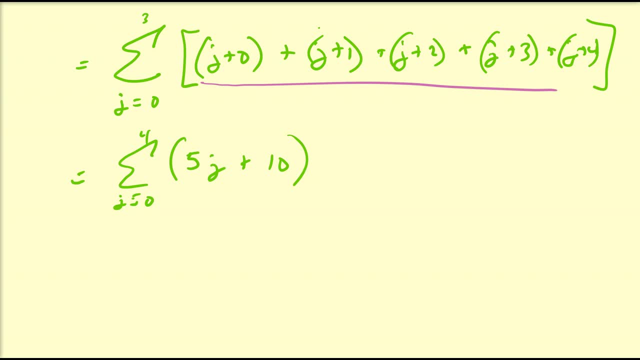 plus three is six, plus four is ten. right, All right. so what can we do? Well, we can replace j with the numbers from zero to four and then add up those expressions. So one way we can do is we can actually distribute the sum, because 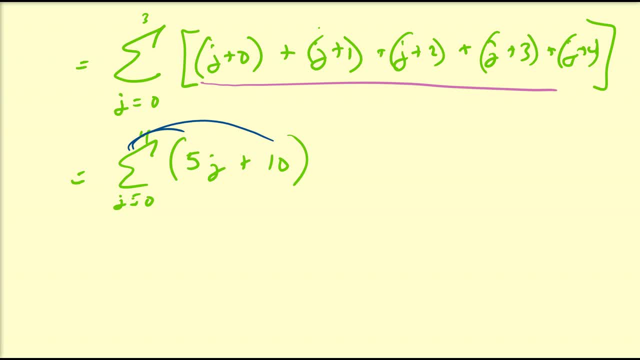 we know sum is commutative over the set of reals, So we can rewrite this instead as the sum from j is equal to zero to four of five. j plus the sum from j is equal to four zero to four of ten, And then we can factor out these constants. 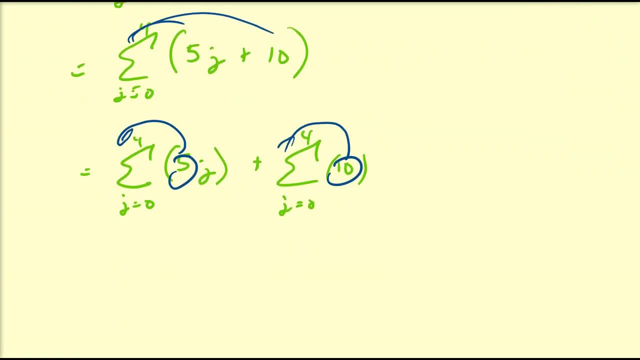 out of the sum, since they're all common terms, And then we're just going to have the sum, or five times the sum from j is equal to zero to four of j, plus ten times the sum from j is equal to zero to four of one. All right, so what is this going to be equal to? So this: 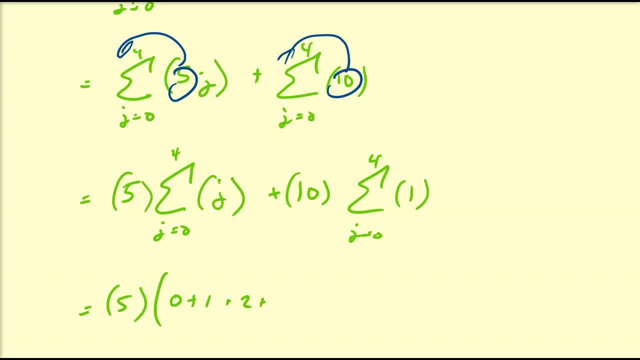 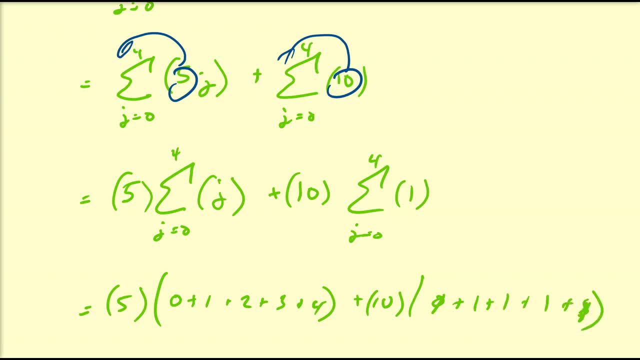 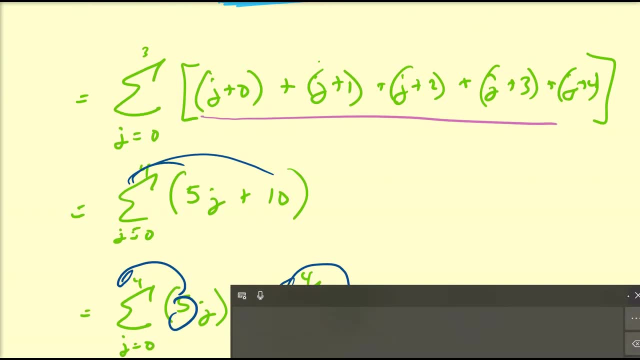 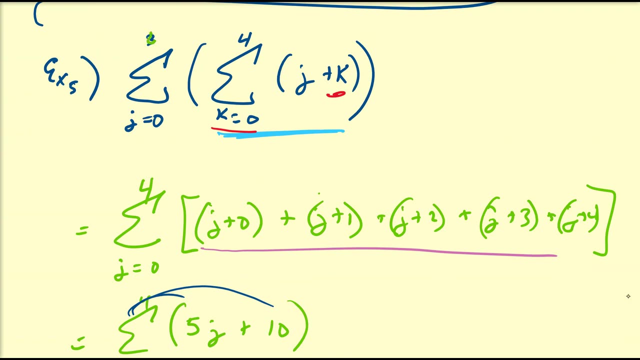 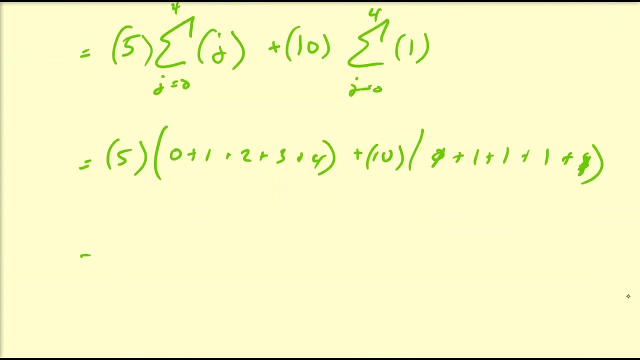 plus three, plus four, plus five different ones. All right, Oh, we started our sum at four, So let's just replace that with four. All right, so now we have this sum, So we're All good, no problem, Alright, so what do we got? 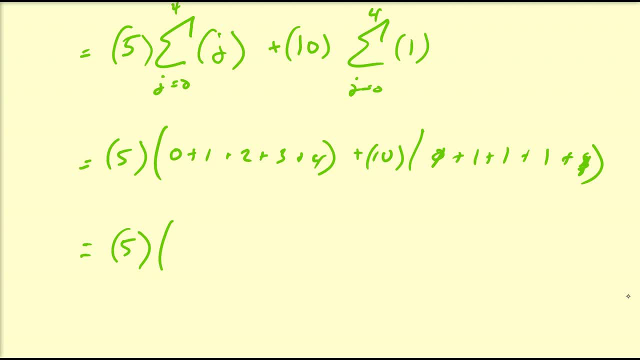 So this is going to be 5 times. so 4 plus 3 is 7, plus 2 is 9, plus 1 is 10, plus 10 times 1, so that's going to be 5.. So we have: 5 times 10 is 50,. 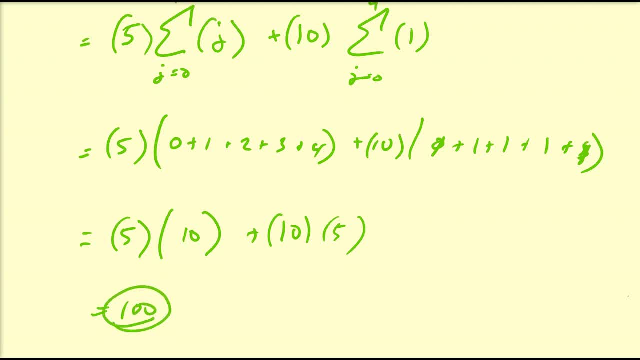 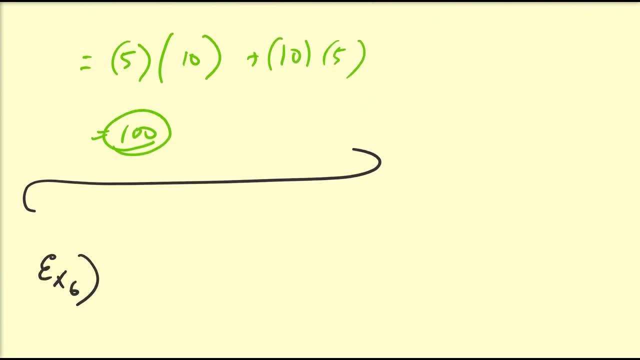 5 times 10 is 50, so this is going to come out to 100.. It's a beautiful sum. So now let us look at the product notation. so example 6.. So this is going to go similarly, so this is going to be the product from k is. 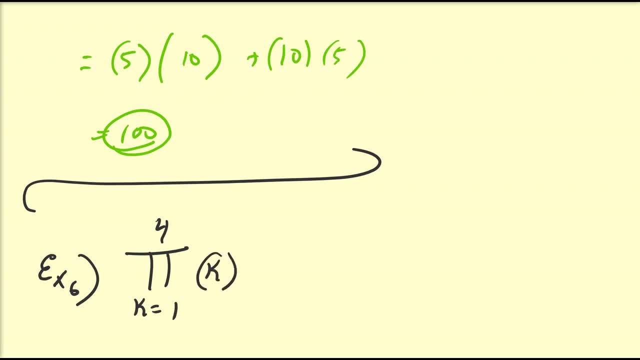 equal to 1 to 4 of the expression k. So we're going to multiply all the numbers k from: k is equal to 1 to 4, so this is going to be 1 times 2 times 3 times 4, so this is going to be 1 times 2 is 2, times 3. 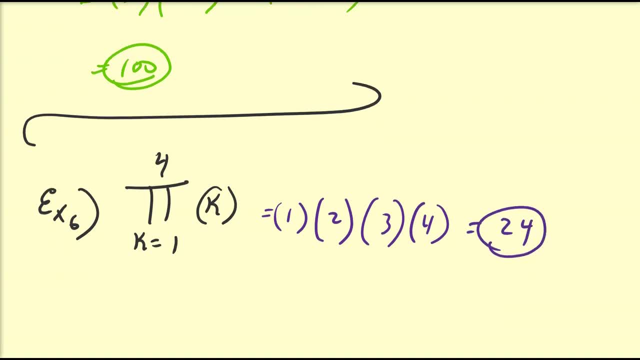 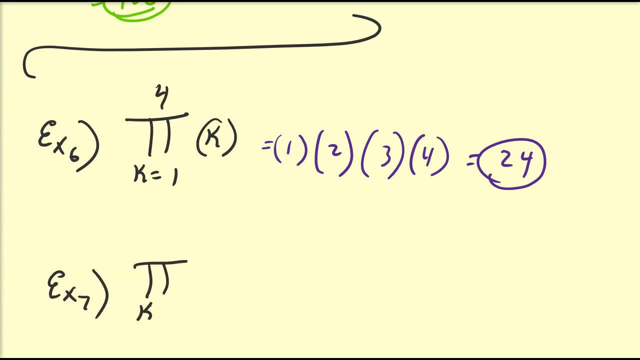 is 6, times 4 is this is going to be 24.. Alright, so another basic example. Let's consider: the product from k is equal to 1 to 4 of 1 over k. So what's this going to be? 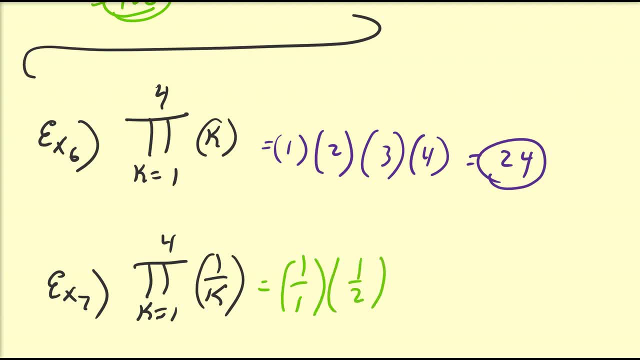 So this is going to be 1 over 1 times 1 over 2 times 1 over 3 times 1 over 4.. And of course, this is pretty much the same as the beginning, just the reciprocal. So that's just going to be 1 over 24.. 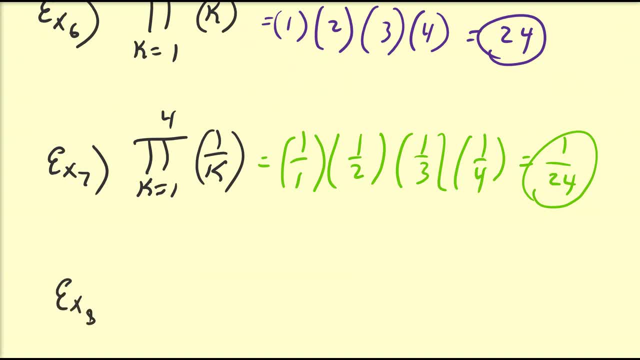 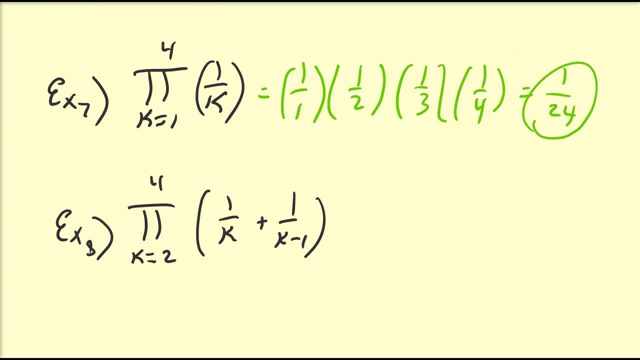 Now let's do something a little bit more fun. Let's do: the product from k is equal to 2 to 4, of 1 over k plus 1 over k minus 1.. So let's replace k with all the numbers from 2 to 4.. So this is going to be. 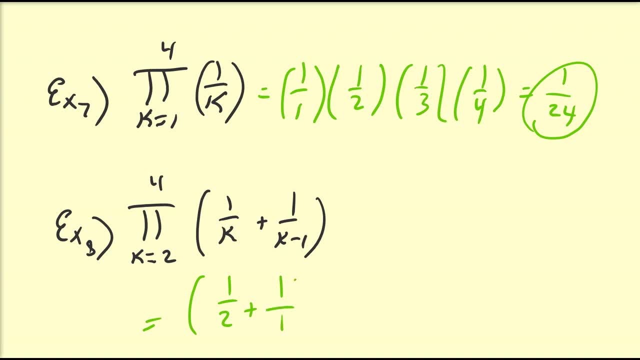 1 over 2 plus 1 over 2 minus 1,, which is 1,. multiplied by 1 over 3 plus 1 over 3 minus 1,, which is 2, times 1 over 4 plus 1 over 4 minus 1, which is 3.. 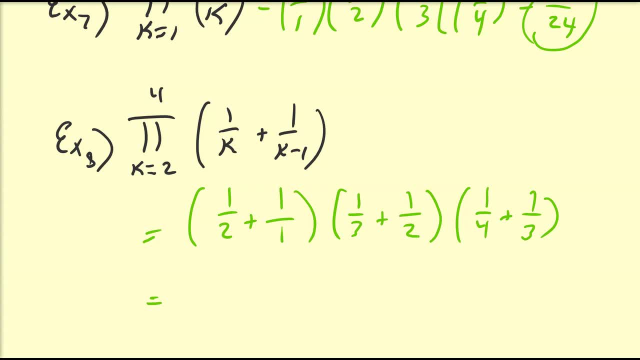 So we know that 1 half plus 1 over 1 is going to be 3 over 2, 1 third plus 1 half is going to be 5 sixths, and 1 fourth plus 1 third is going to be 7 twelfths. 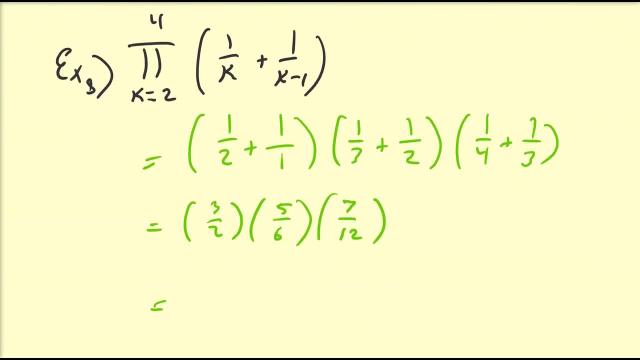 So we know that 3 times 5 times 7 is going to come out to 105, and 2 times 6 times 12 is going to come out to 144.. We notice that the sum of the digits is divisible by 3, so we can divide top and bottom. 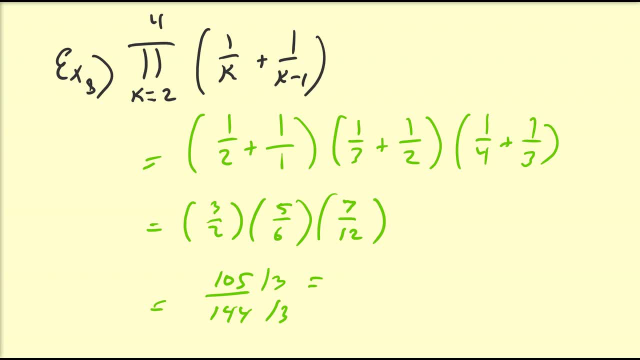 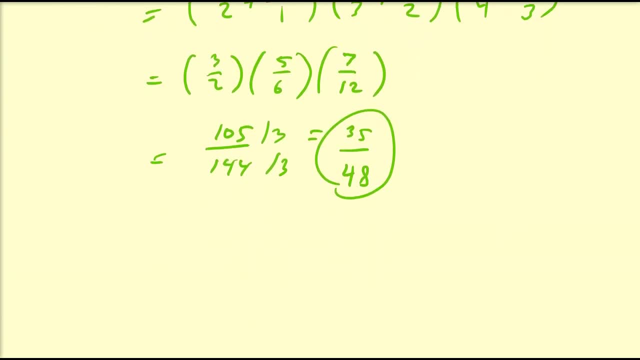 by 3 to simplify. So this is going to reduce down to 35 over 48.. Alright, so let's just do one more example just to review these concepts. So let's calculate: the sum from j is equal to 0 to 3 of the product. 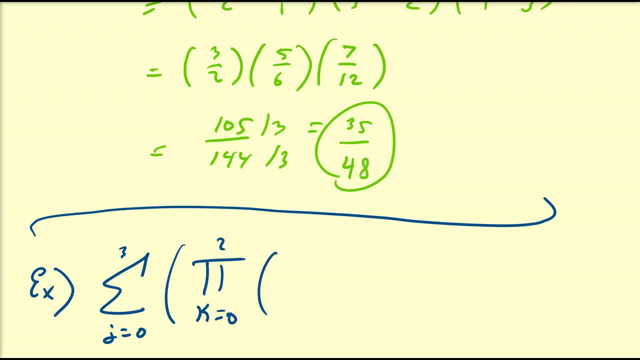 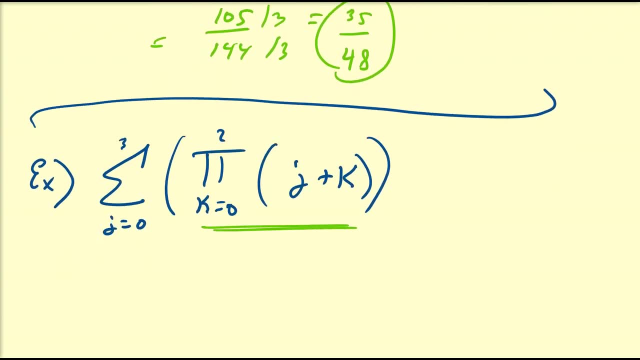 from k is equal to 0 to 2 of the expression j plus k. So we'll start with this inner product here. So this is going to be equal to the sum from j is equal to 0 to 3 of. so we're going to multiply these expressions and replace k with all the numbers from 0 to 2.. 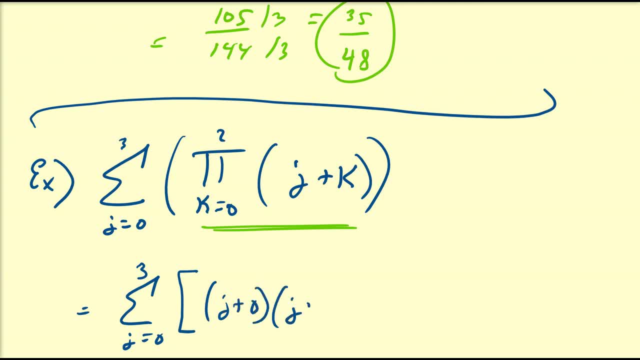 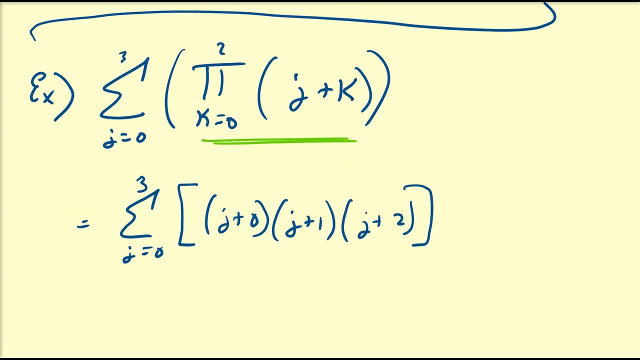 So this is going to be j plus 0 times j plus 1 times j plus 2.. And what we can do is we can triple expand this expression, So we can do j plus 0 times j plus 1, or just j, since plus 0 doesn't. 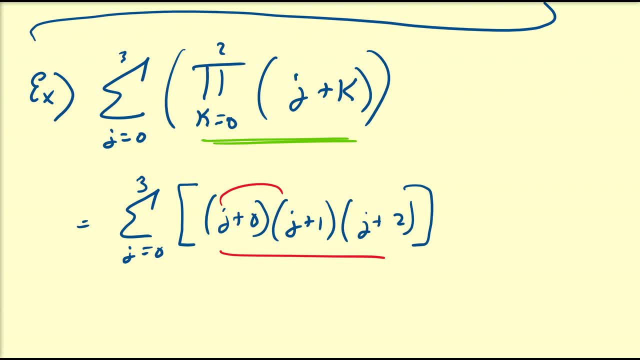 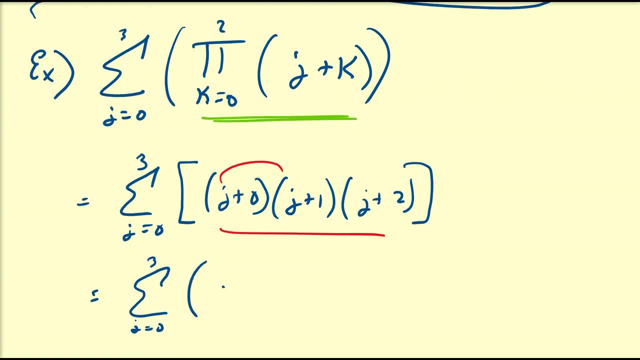 really do anything. So once we expand this expression, one can find that that's going to come out to j, to the fourth No, So this is going to be j squared. let's see 2j, 3j, so 3j. 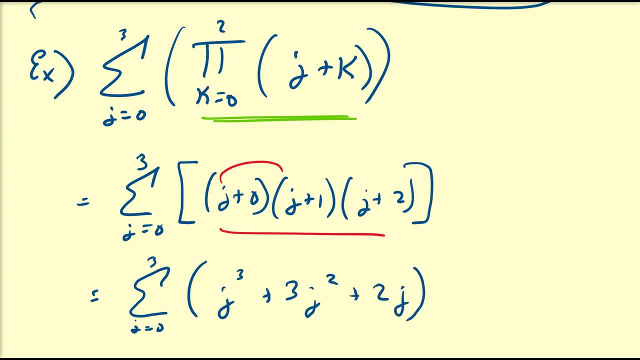 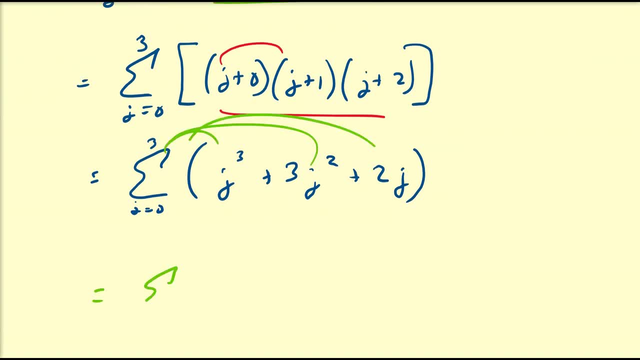 squared and then plus 2j. So then we're going to distribute the sum over each of these, just to make this a little bit easier. So this is going to be: the sum from j is equal to 0 to 3 of j, cubed. 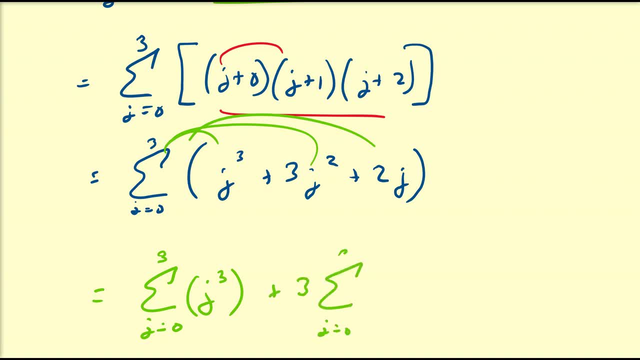 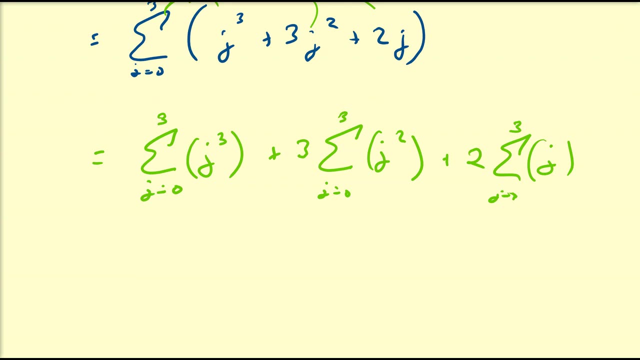 plus 3 times the sum from j is equal to 0 to 3 of j squared. plus 2 times the sum from j is equal to 0 to 3 of just j. Alright, so notice that j is equal to 0 for j cubed, j squared and j is just 0.. So we can actually 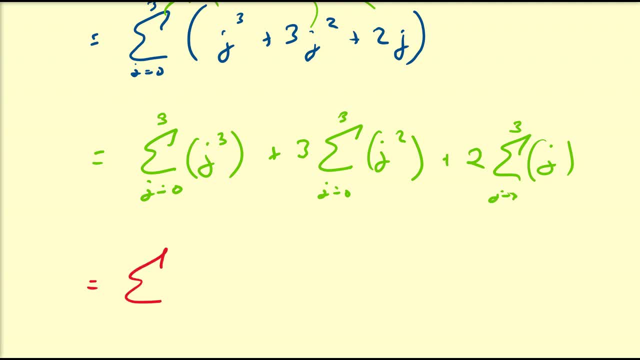 just simplify this and rewrite this in a more nicer way. So we can just rewrite this as just: the sum from j is equal to 1 to 3 of j. cubed plus 3 times the sum from j is equal to 1 to 3. 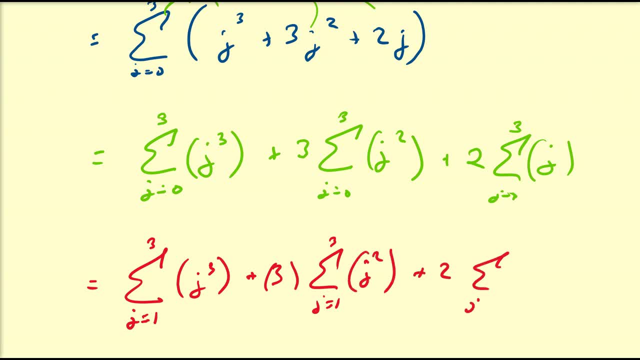 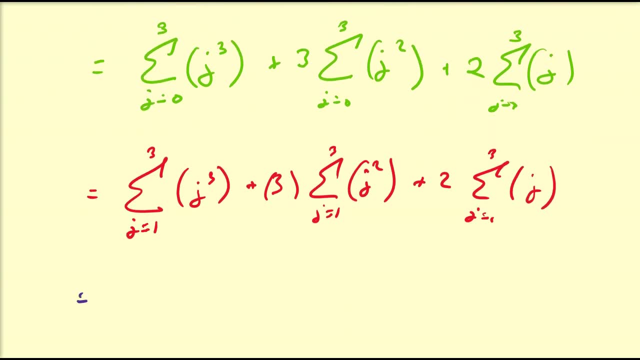 of j squared plus 2 times the sum from j is equal to 1 to 3 of just j. Alright, that makes it a little bit more nicer to write. Then we don't have those zeros floating around. So this is going to be 1 cubed plus 2 cubed plus 3 cubed. 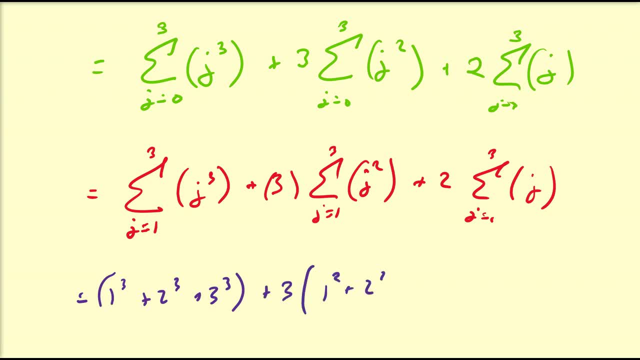 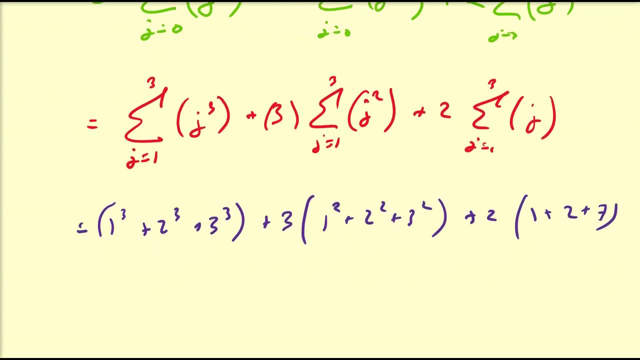 in the first term, plus 3 times 1 squared plus 2 squared plus 3 squared in the second term, plus 2 times 1 plus 2 plus 3 in the third term. So this is going to be equal to 1 plus 8 plus so 3 times 3. 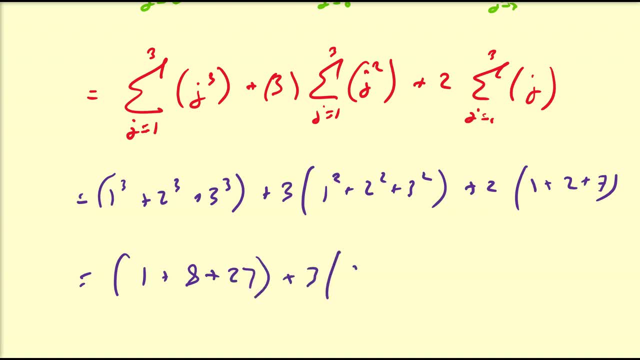 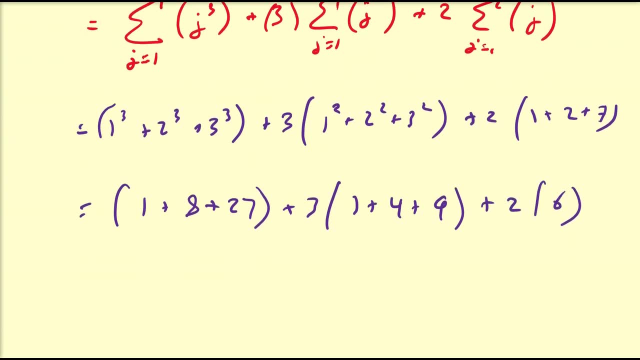 is 9 times 3 is 27 plus 3 times 1 plus 4 plus 9 plus 2 times 1 plus 2 is 3 plus 3 is 6.. Alright, so we have 27 plus 1 is 28 plus 8 is 36 plus. 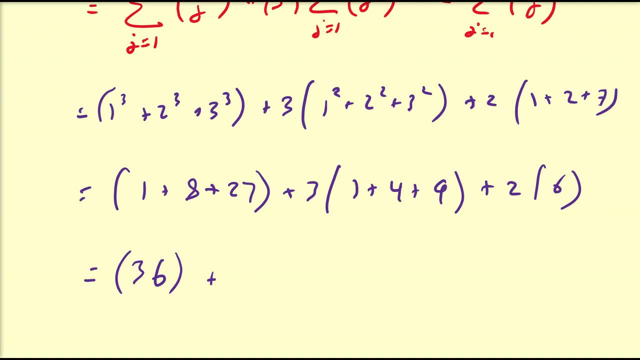 let's see: 1 plus 4 is 5, plus 9 is 14, and 14 times 3 is going to come out to 42, and then 2 times 6 is 12.. Alright, so what do we have here? So 2 plus 2 is 4 plus 6 is. 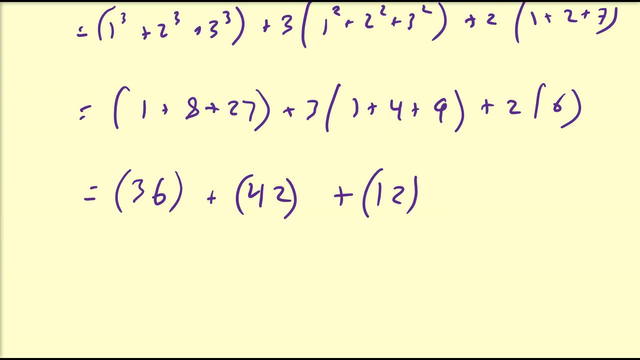 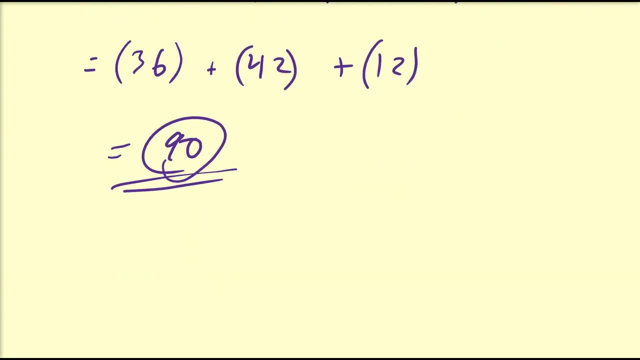 going to add up to 10.. 3 plus 4 is 7, plus 1 is 8, so this is going to come out to 90.. So this is just a basic overview of how to use these notations, namely sigma and pi. Sometimes, if you see the same sums. 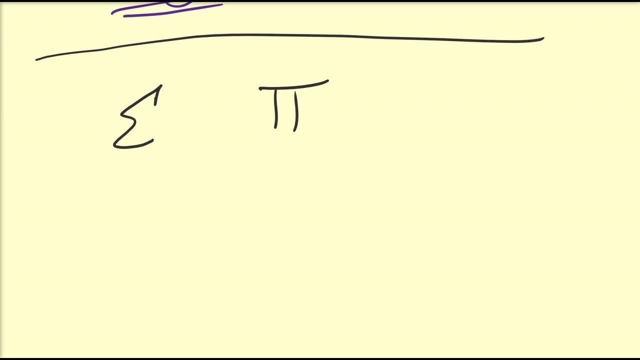 with lower limit and upper limit. you may just see people just express expressions like this, you know, without actually writing the limits. but that should be a well defined thing and it should be stated in whatever literature you're reading. And if you see, not a finite number here, but 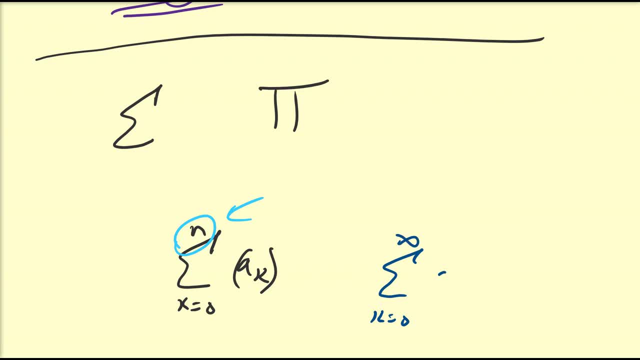 something like: the sum from k is equal to 0 to infinity of some expression. this is called an infinite sum, and the same thing can go for a product. We'll discuss these at a later time when we have a couple more details underneath this. Hope you enjoyed. 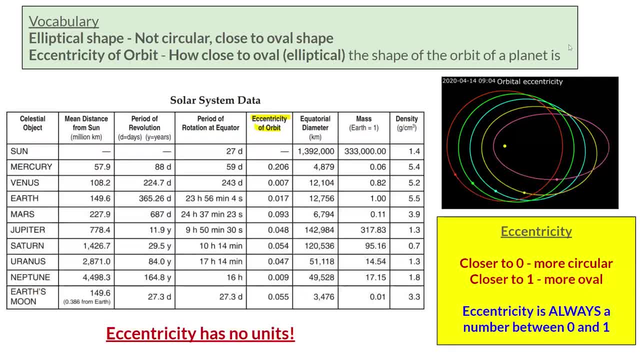 Hey guys. so today we're going to talk about the eccentricity of a planet's orbit. So let's talk about a few vocabulary words. The first is elliptical. Elliptical is a term we use to describe the shape of a celestial object, and in this case we're talking about the orbit of a.